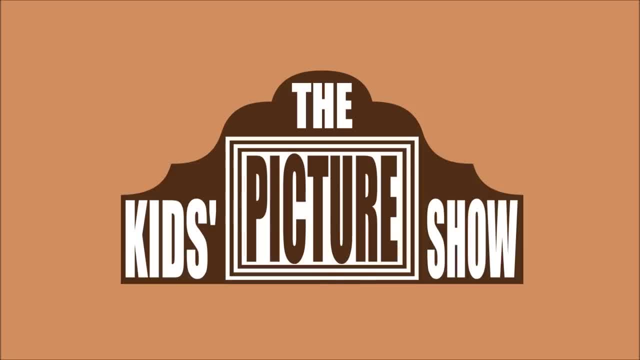 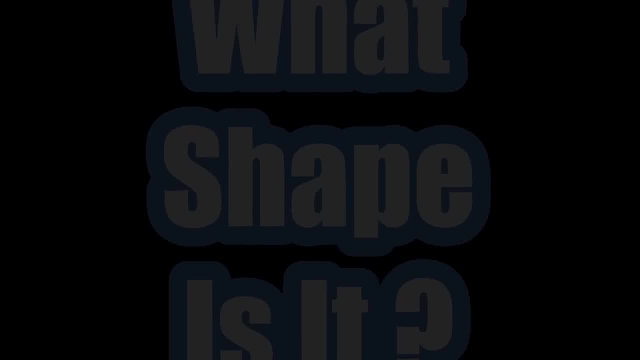 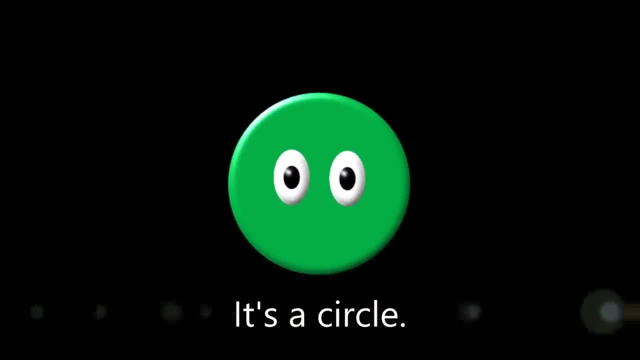 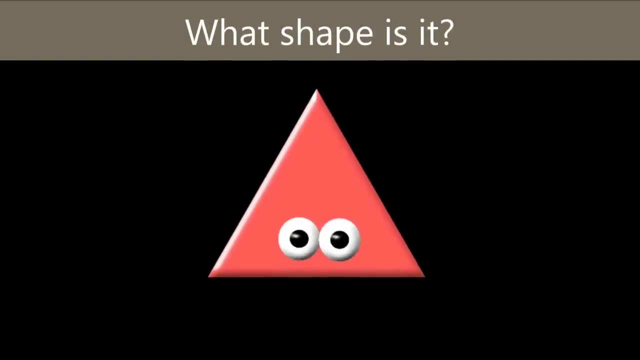 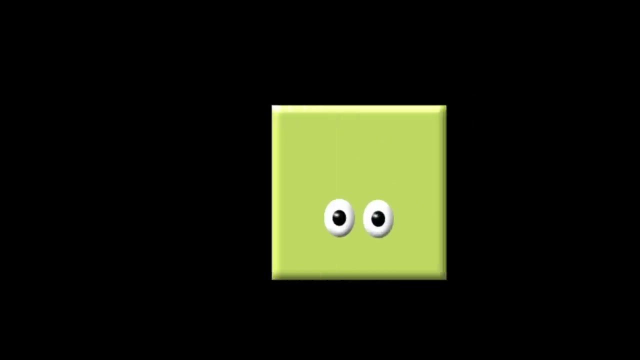 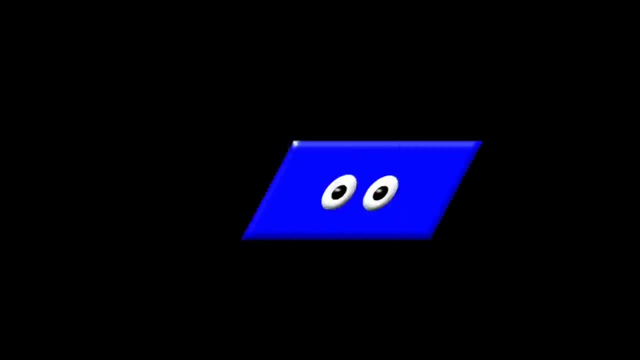 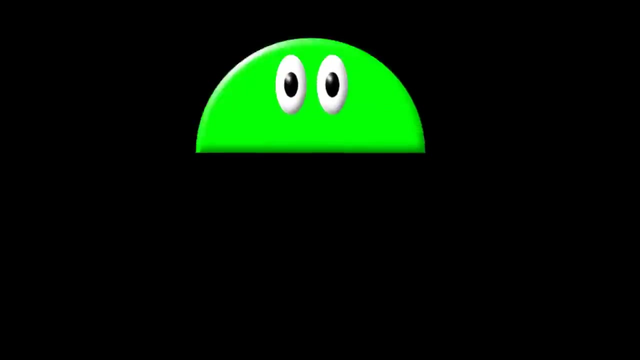 What shape is it? What shape is it? It's a circle. What shape is it? It's a triangle. What shape is it? What shape is it? It's a square. What shape is it? It's a rectangle. What shape is it? 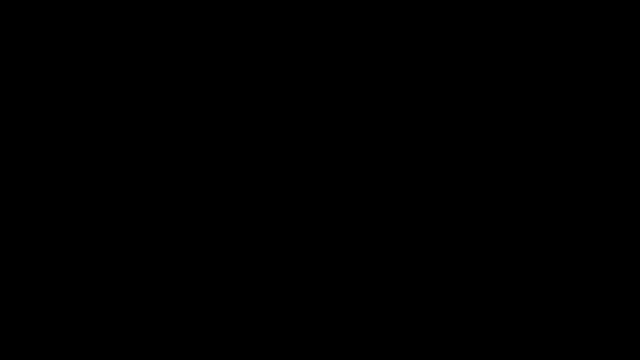 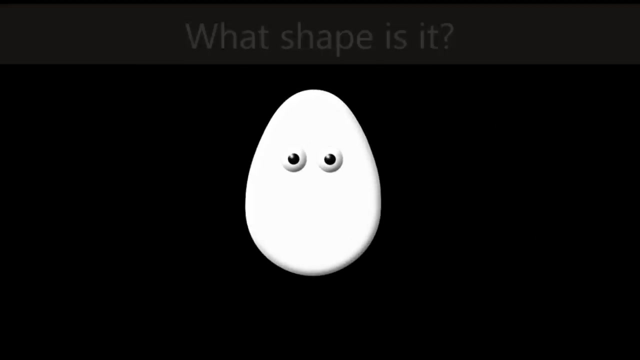 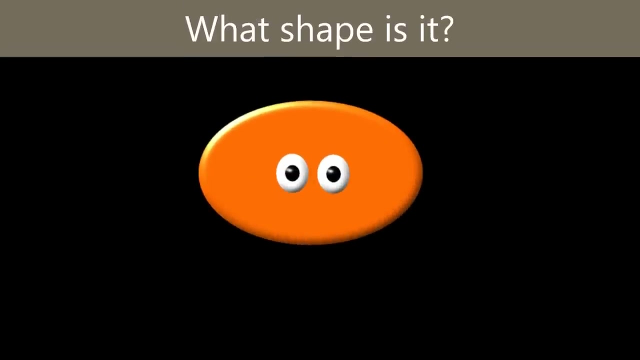 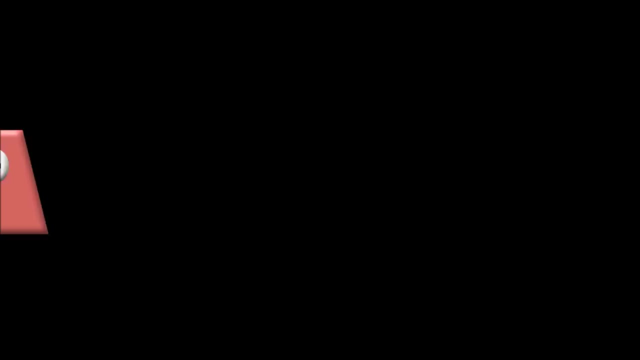 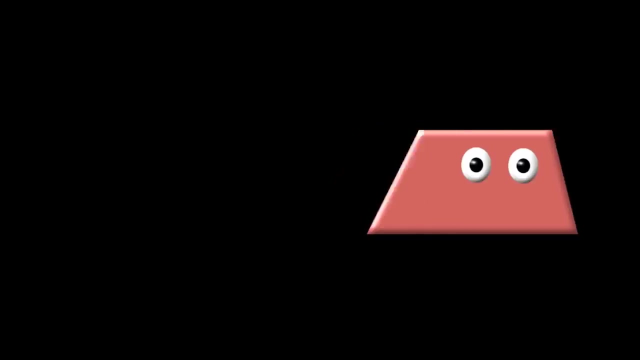 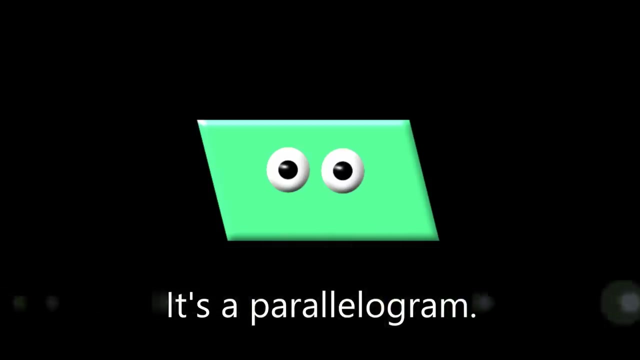 It's a semicircle. What shape is it? It's an oval. What shape is it? It's an ellipse. What shape is it? It's a trapezoid. What shape is it? It's a parallelogram. 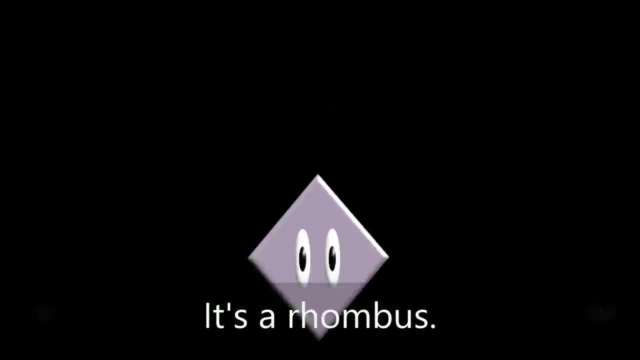 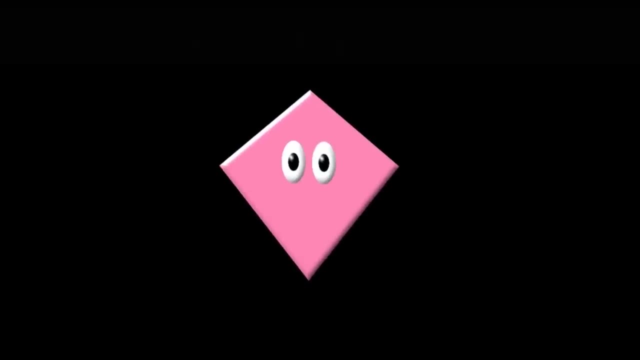 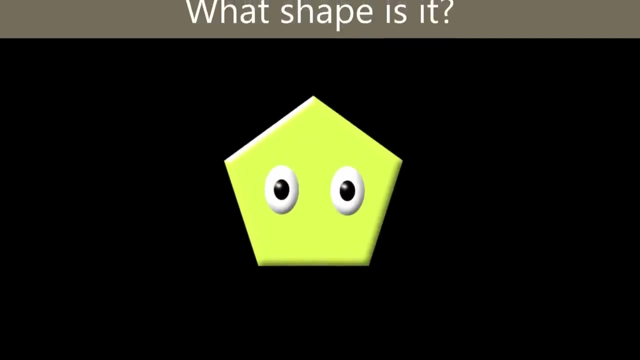 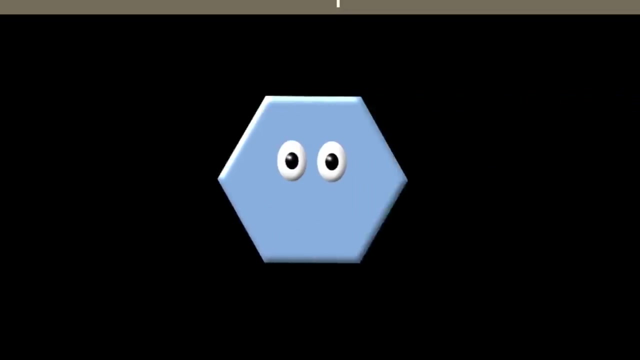 What shape is it? It's a rhombus. What shape is it? It's a kite. What shape is it? It's a pentagon. What shape is it? It's a hexagon. What shape is it? It's a hexagon. 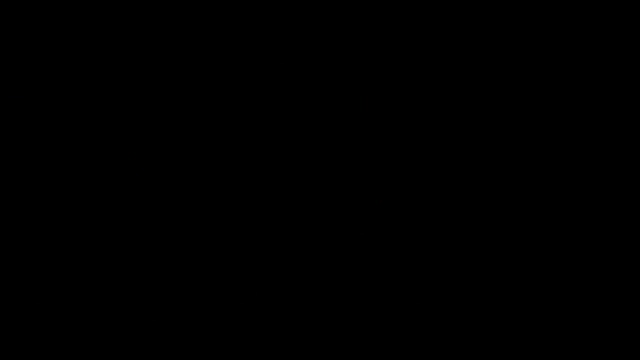 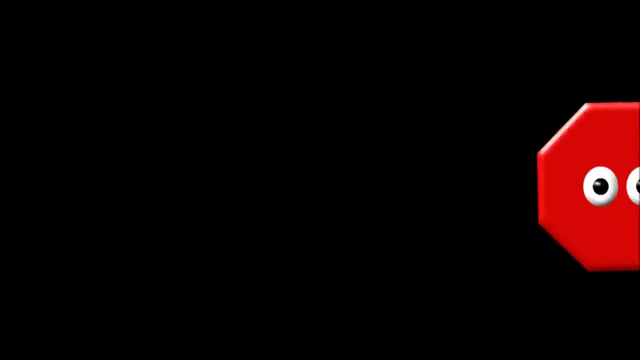 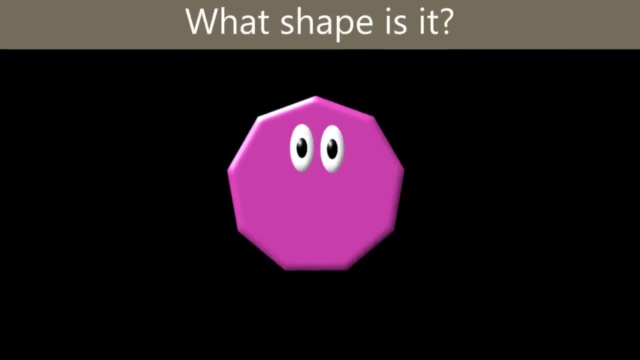 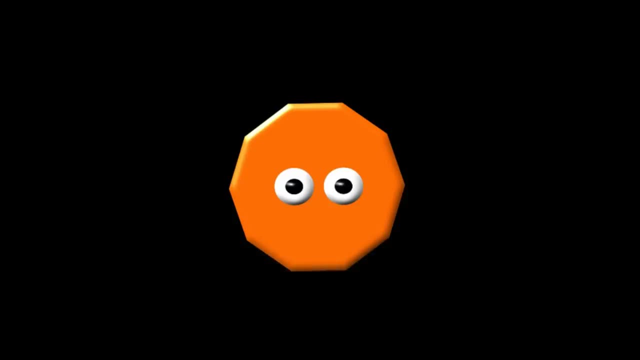